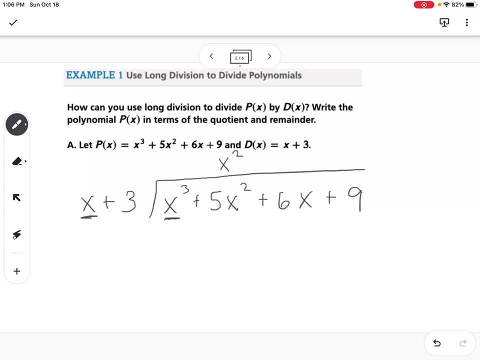 with the correct place value. So x squared goes above the 5x squared because they have the same power of x. Now you take the number that you're the term that you put up above, and you're going to multiply it by the divisor. So this would be x squared times x. 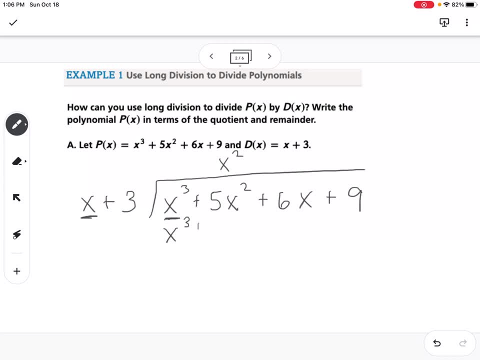 gives me x cubed and x squared times 3 gives me 3x squared. Then my next step is to subtract, So the x cubes cancel. 5x squared minus 3x squared is 2x squared, And then I bring down the. 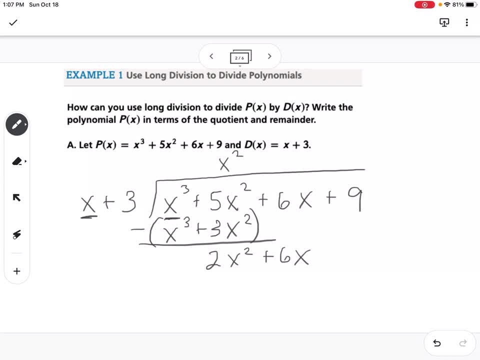 plus 6x. Now I say x. So again I'm looking right here. x goes into 2x squared. How many times 2x? So I'm going to add plus 2x, Then I'm going to multiply 2x times x. 2x squared 2x times 3 is 6x. We're going to subtract. 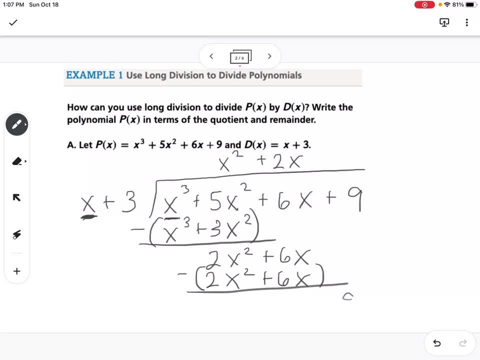 And we get 0. They both cancel, So then we just bring down the 9.. Well, x cannot go into 9.. So therefore, that means that 9 is our remainder, And the way that we write this is so we have x. 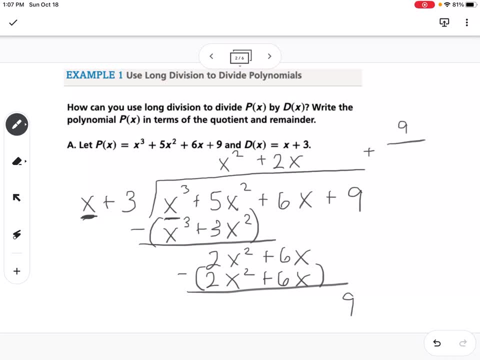 squared plus 2x and then we write 9 over our divisor, which is x plus 3.. So this whole answer up here is our quotient, So the answer to our division problem. So again, dividend is the part that goes underneath, Divisor is the part out here. Remainder is our, whatever we have left. 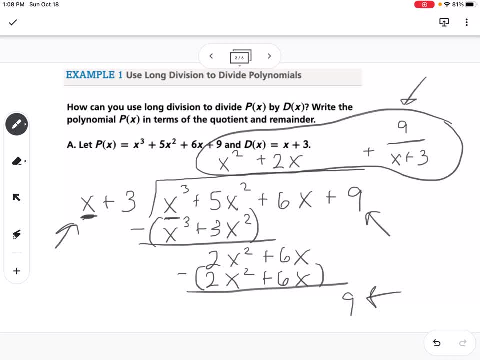 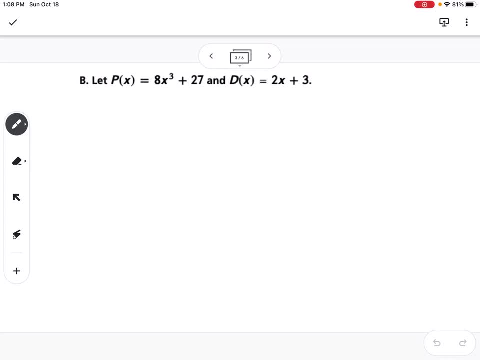 over. And then this is the quotient. Okay, So here's another example. So this one p of x is 8x cubed plus 27.. And d of x is 2x plus 3.. So you'll notice, on this one, when I go to write the dividend, I have 8x cubed. I'm missing an x. 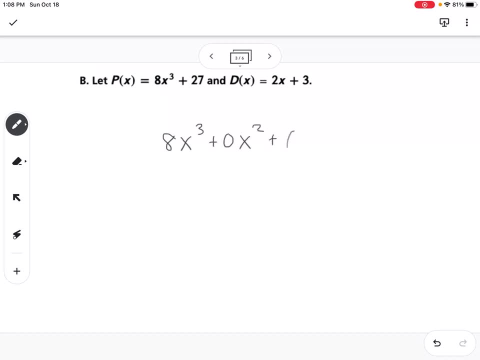 squared, So I'm going to put 0x squared. I'm missing an x, So I write 0x And then I write 27.. So this is an example of where I was missing terms. So you need to put 0 in there as a. 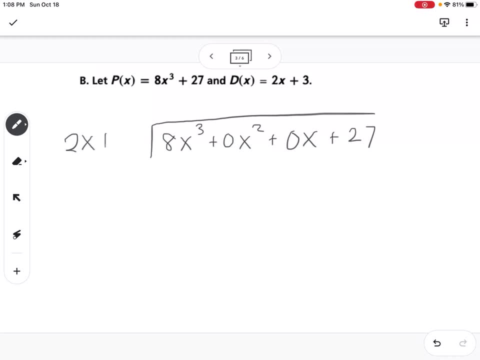 placeholder. Okay, And then my divisor is 2x plus 3. Okay, So we say 2x times what gives me 8x cubed, And that would be 4x squared. So I line it up with the x squareds, Then I multiply, I get 8x cubed. 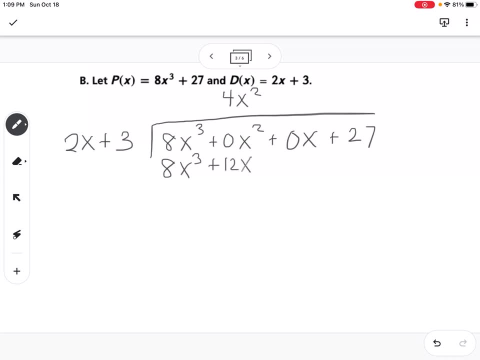 4x squared times 3 is 12x squared. Then I subtract And I get negative 12x squared. I bring down the 0x 2x times what gives me negative 12x squared. That would be minus 6x. Then I multiply, I get. 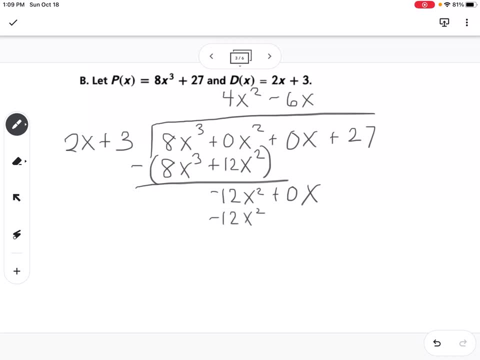 negative 12x. squared Negative 6 times 3 would be minus 18x. Subtract That becomes positive 18x. I bring down the plus 27.. 2x times what gives me 18x. That would be 9.. 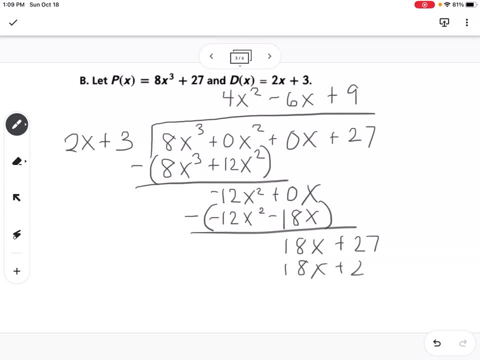 9 times 2 is 18x, 9 times 3 is 27.. And when we subtract we get 0.. So this one doesn't have a remainder. So this- and we'll talk about what that means in a couple examples here- So that one does not have a remainder. So my answer, my quotient would just be 4x squared minus 6x plus 9.. 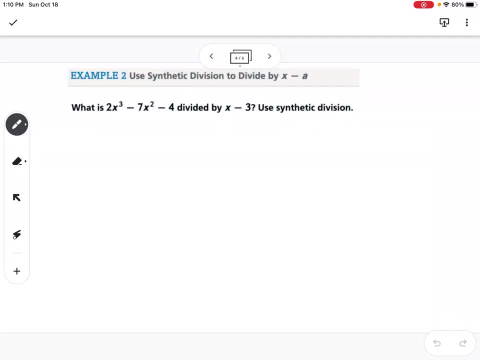 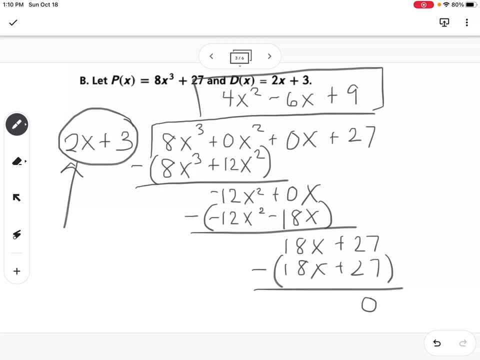 Okay, Okay. Example 2 is now using a different type of division. It is using synthetic division. So the previous two examples we did, we actually could have used synthetic division. So you're not able to use synthetic division if you have a divisor. so, like this part right here, that is a higher power than a linear function. 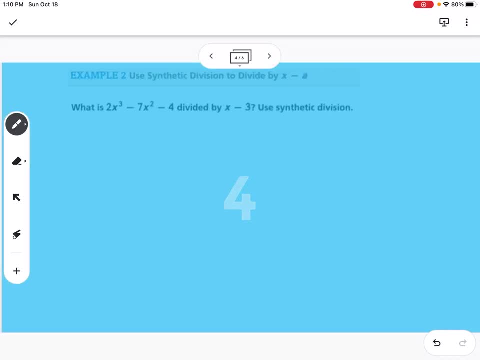 So if it's a linear function that you're dividing by, you can use synthetic division, But if it's squared or cubed, you would need to use long division. So a lot of people say, well, once I show you synthetic division, you're going to say: this is so much easier. 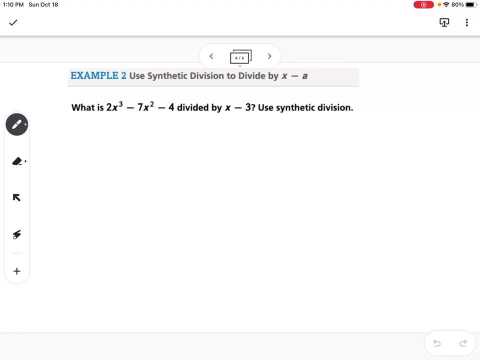 And so the answer to when you can use each one is dependent on what the divisor is. Okay. So how we set up synthetic division is: we're going to put numbers on the inside that correspond to the coefficients of your dividend. So we're going to write 2, negative 7.. Notice, I'm missing an x term. so I'm going to put 0, and then negative 4.. 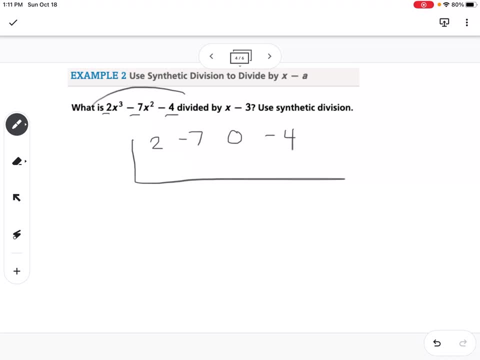 So those represent the coefficients. So we're going to put the coefficients of my dividend right here. Okay, Now this is my divisor and that's going to tell me what number, what k value, I'm going to put on the outside of this. 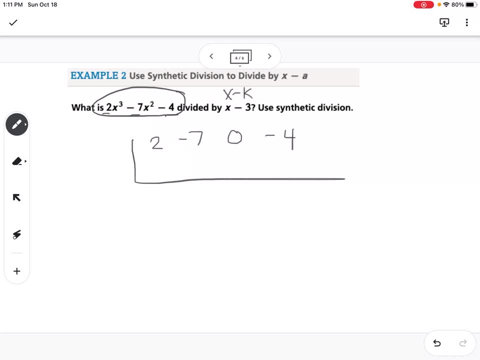 So this is x minus k, So our k in this case is 3.. So we're going to put a 3.. The other way to think of the number out here is what makes the divisor equal 0.. So it's kind of like a factor. 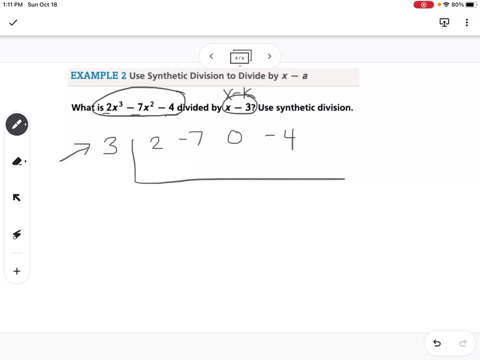 So you're saying x, x minus 3, what makes that equal 0? Just plain positive 3.. Okay, So now how you do synthetic division is you're going to add straight down? So, on the 2, we're going to just drop the 2 straight down. 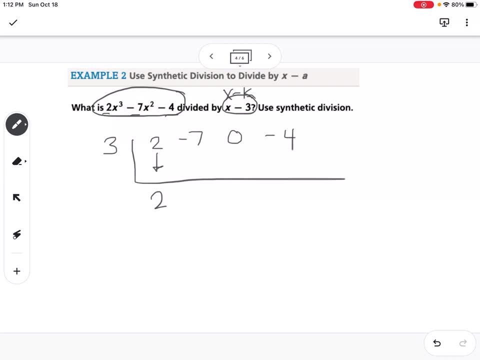 And then you're going to multiply by the k value. So 2 times 3 is 6. And I'm going to put that number right here. Now I'm going to add straight down: So negative 7 plus 6 is negative 1.. 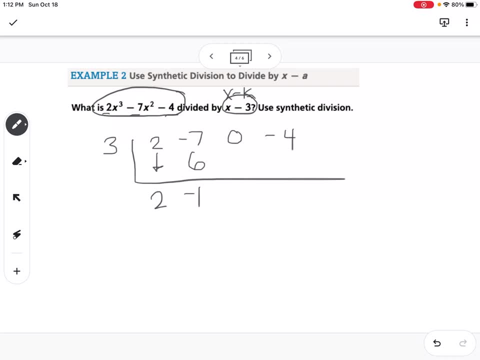 Now I'm going to multiply by the k value. So negative 1 times 3 is negative 3.. I'm going to write it right there, Then I'm going to add down. So this would be negative 3.. Then negative 3 times 3 is negative 9.. Then negative 4 plus negative 9 is negative 13.. 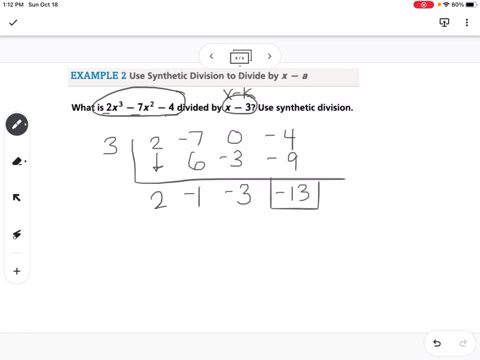 And when you get to that last number, I always like to put a box around it because that represents our remainder. So it always helps me separate that final number from the rest of the equation. So if you have a cubic like this and you're taking, you're dividing by a power of x, that means your answer is going to be negative 3.. 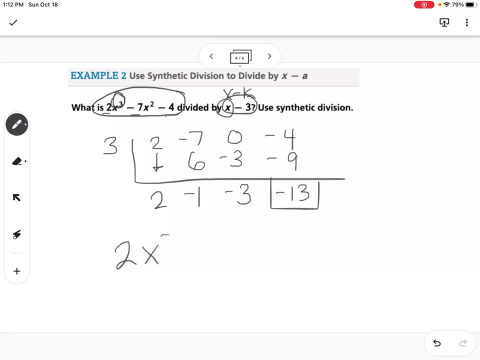 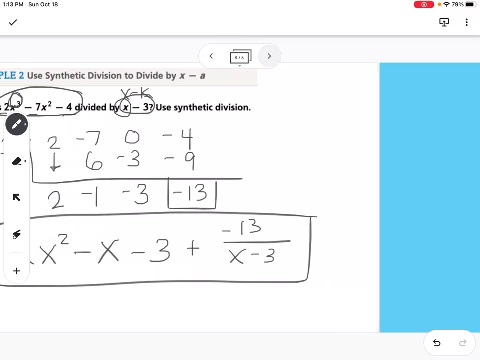 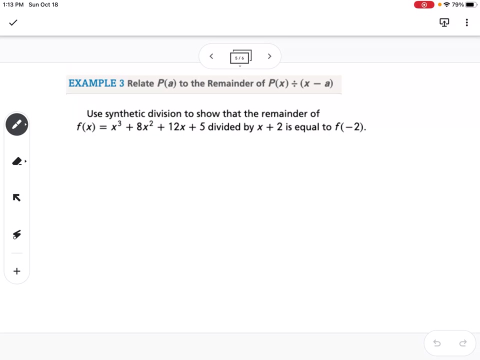 So this would turn into 2x squared minus x minus 3, plus negative 13 over x minus 3.. So that would be my final answer. Okay, So example 3 is talking about the remainder theorem. So the remainder theorem says that if you do synthetic division and the remainder you get is going to be negative 3.. 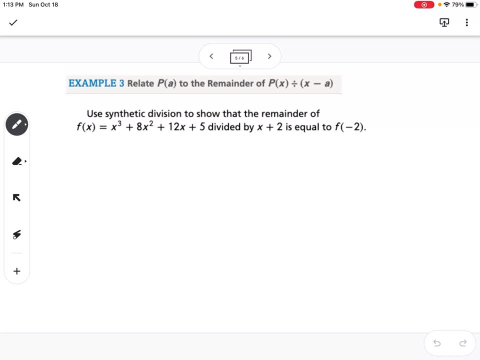 So that would be my final answer. So example 3 is talking about the remainder theorem. So the remainder theorem says that if you do synthetic division and the remainder you get is going to be negative 3.. So that would be my final answer. So example 3 is talking about the remainder theorem. So the remainder theorem says that if you do synthetic division and the remainder you get is going to be negative 3.. 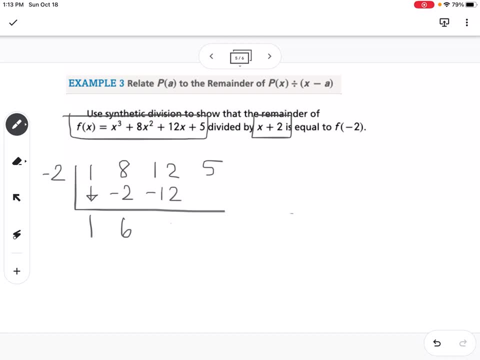 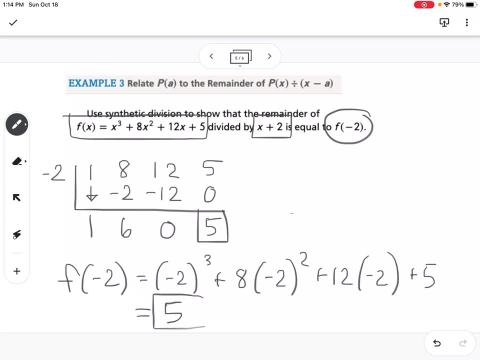 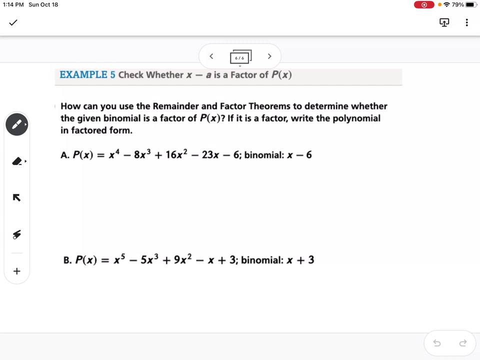 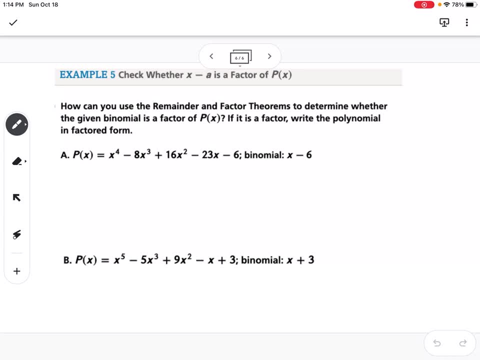 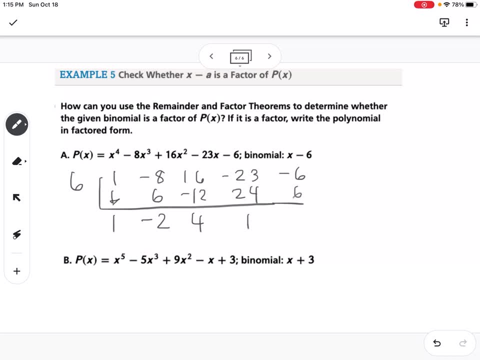 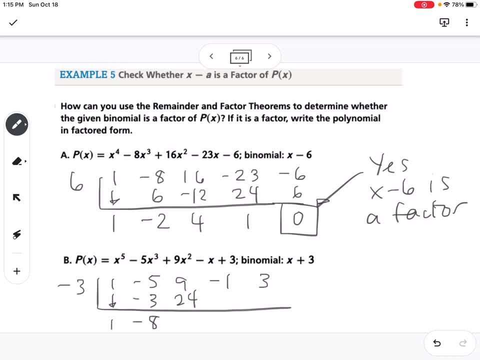 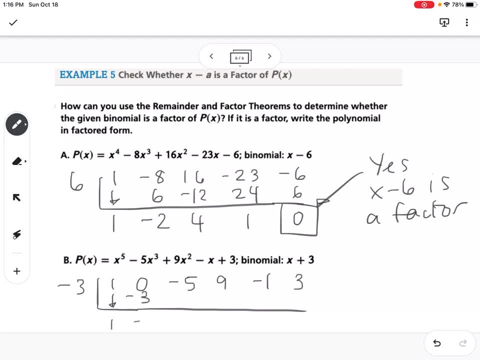 Okay, so this would be negative 3,, this would be 9,, so that would be 4, negative 12, negative 3, 9, so 8, negative 24, so our remainder would be negative 21,, which means no, it's not a factor.